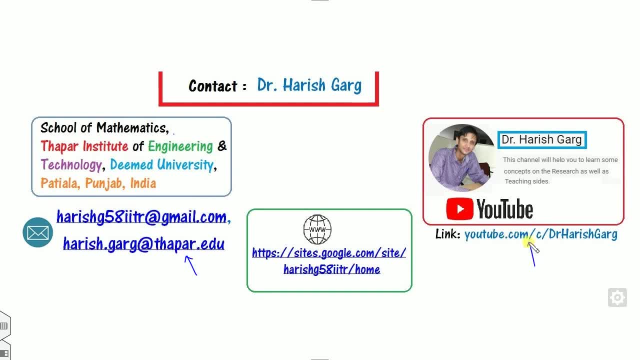 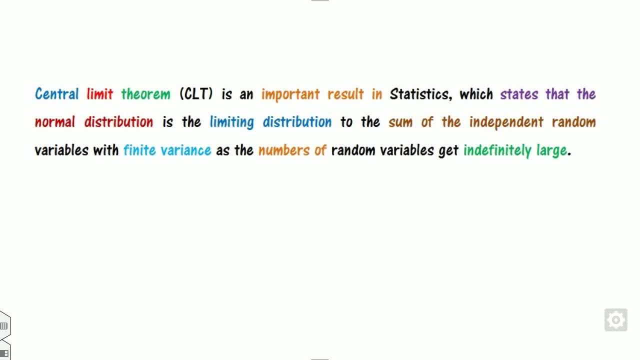 You can contact me. either of my email ids are there or you can simply follow this, my channel, Dr Harish Garg, on the YouTube. you can find the various videos related to probability and stat. First of all, what is the central limit theorem and why it is so important? 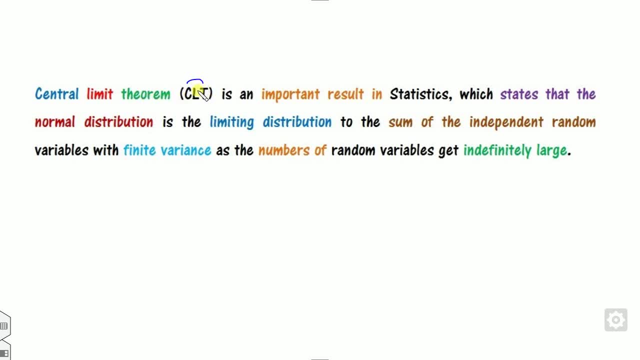 What is the central limit theorem? It is abbreviated as a CLT and it states that the normal distribution is just the limiting distribution of the sum of independent random variable. Make sure that the random variables are independent and having the finite variance. So also you can see this is a random variable, So it may be the discrete or continuous is there? 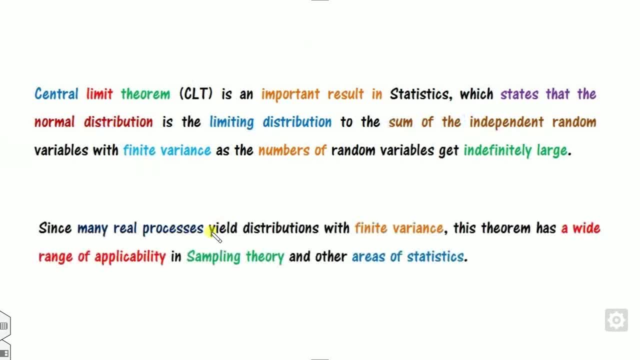 So there is no restriction on the random variable. Also, you can see, this CLT, that is, a central limit theorem- is widely applicable in the sampling theory because all of you know, when we discuss that, the testing of the hypothesis, then we always use the central limit theorem for 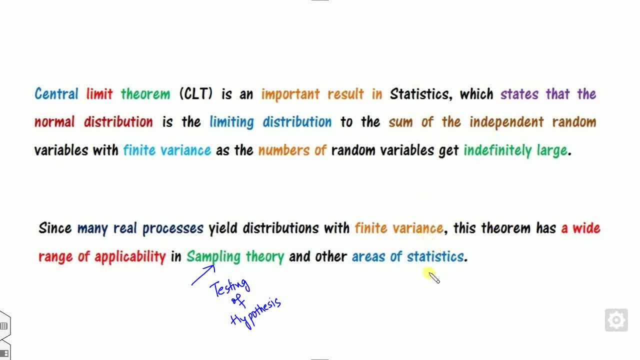 finding the population means from the help of the sampling mean, as well as some and other area of the statistics, like, say, when you discuss about their testing. as well as the sampling is there, What is the central limit theorem suggests to us that, if I say if xi's are, 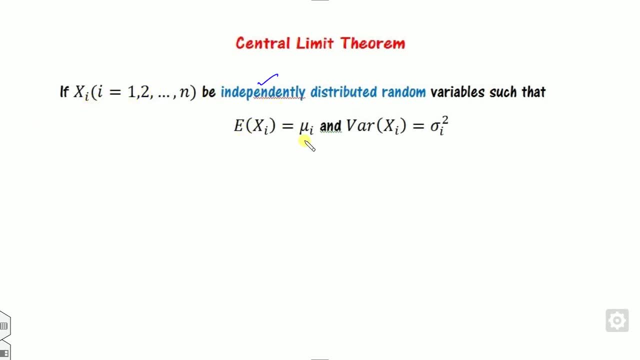 my independent random variables, such that each of the xi's has mean mu, i and the variance is sigma square, then this central limit theorem suggests that as n approaches infinity, that means if I say infinite number of the random variables, then the sum of these random variable denoted as a sn, 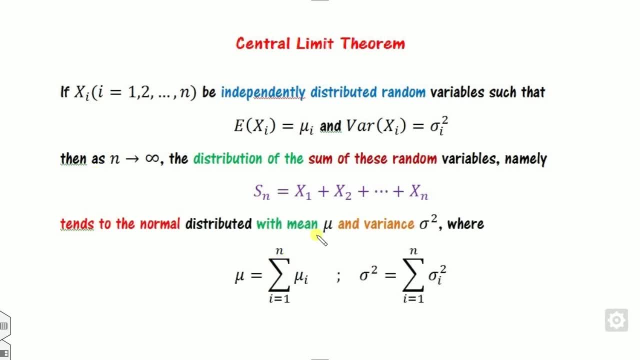 this sn follows the normal distribution with mean of these variances is nothing but the sum of them. So this is the central limit theorem. make sure that n is infinite, but remember infinite means is a very large number in terms of statistics is a very large number. So then the sum of the random variable will follows the. 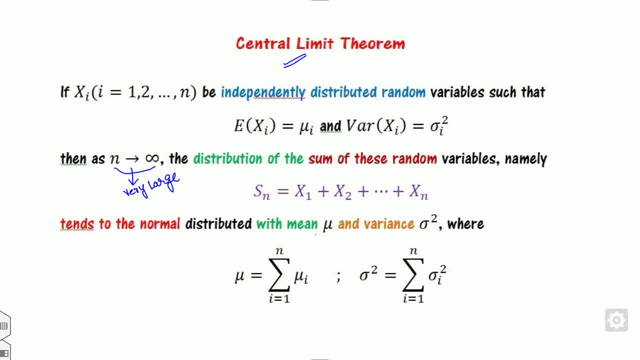 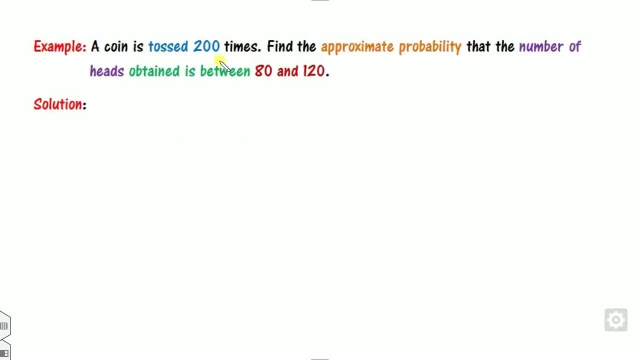 normal distribution. So how we can see in terms of the numerical example we will see. we will discuss 4 to 5 example in this lecture. Let us see here what is given to you. look at that. n is a coin is tossed 200.. So n is a coin is tossed 200.. So n is a coin is tossed 200.. So 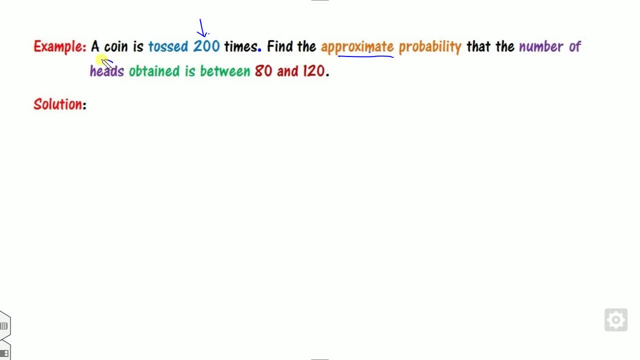 n is a coin is tossed 200.. Now what we can see in this example is technique shelters. you can see we need to useinte verb经 finger or simple to形 how we can to write in terms of 80, then plus is 81, and so on, plus up to 120. so that's not an easy task, because 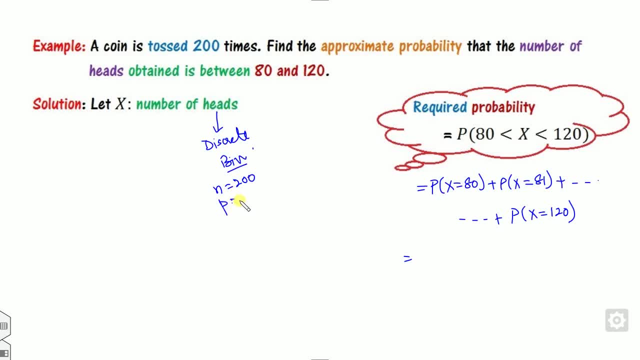 if you apply the binomial distribution, n is my 200. what is the probability of? the head is half, so you can apply here as: n, cx, p raised to power, x, q raised to power, n minus x. so this this is 1 by 2 raised to power 80, 1 by 2 raised to power 120 plus so on, and up to the last one is there. so 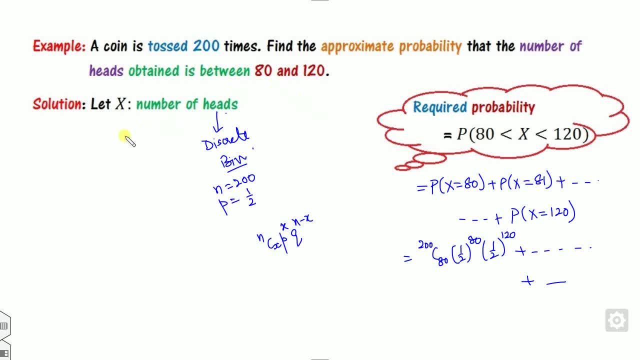 that's not an easy task to calculate them but, in case, by using the center limit theorem, we can approximate the result of them now, since n is very large, so we can apply the center limit theorem. so what we will follow in this lecture will be apply the same theory that we will discuss. 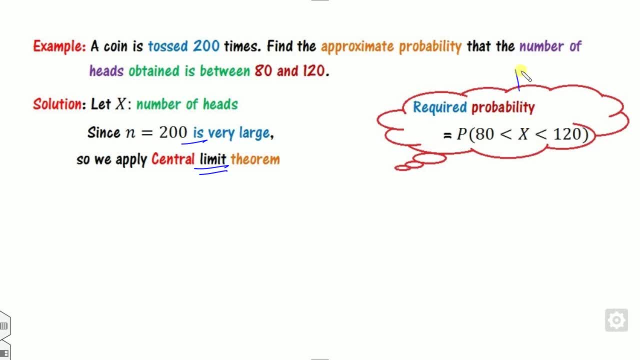 question number one: to the end of them, what we do, we will find what is the required task. then, whatever i have written here, i my task is to calculate the mean. my task is to calculate the variance of this variable. now here is x. x is my number of the head. what is the probability of the head is half, so this is: 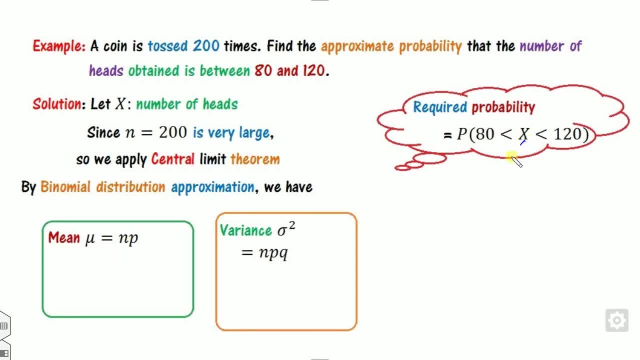 there. so therefore, you can apply the binomial distribution. you have to find the mean and the variance of this, so you can substitute the value of n here. what is the p is probability of the head, so you can find the mean, and the variance is here. therefore, once you will find the mean and variance, 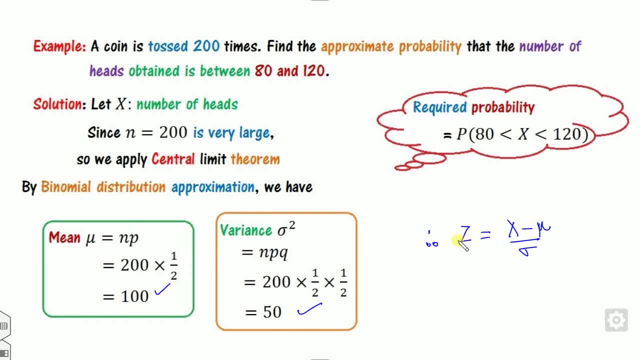 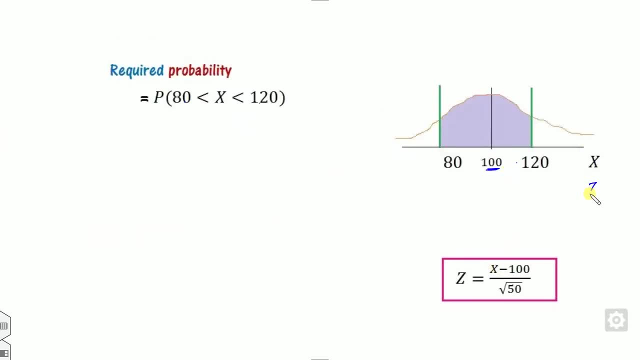 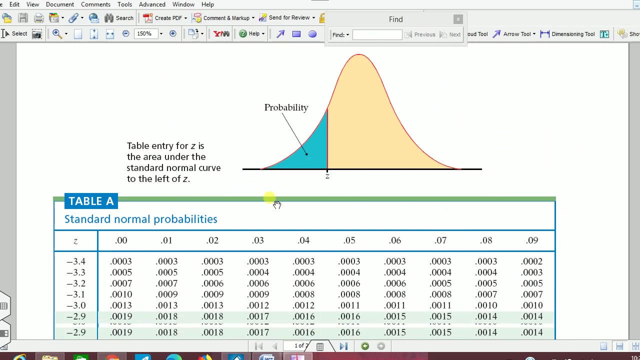 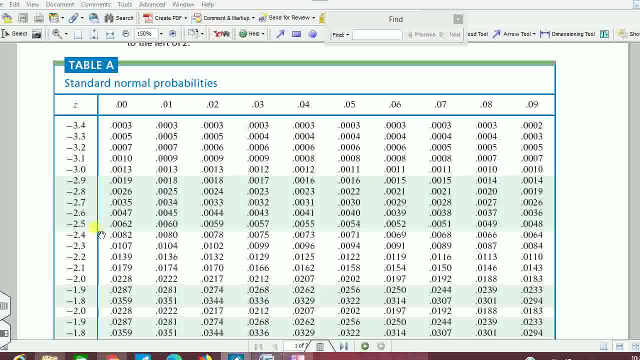 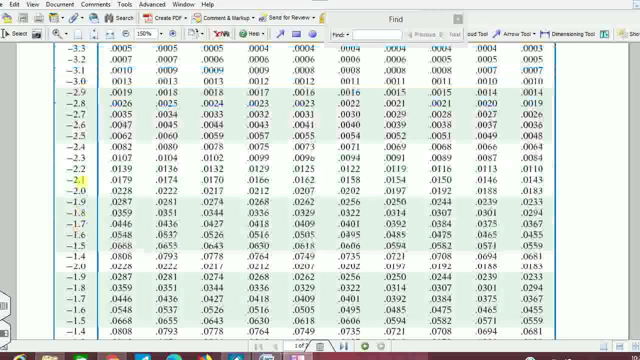 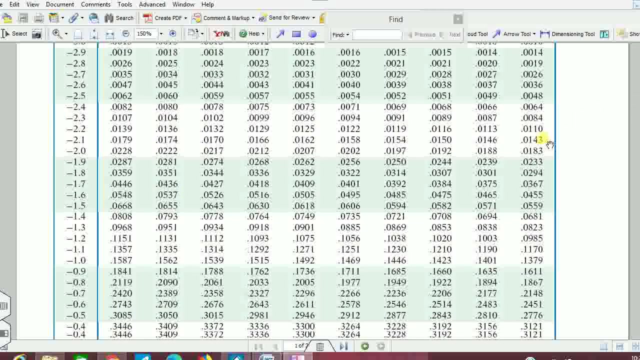 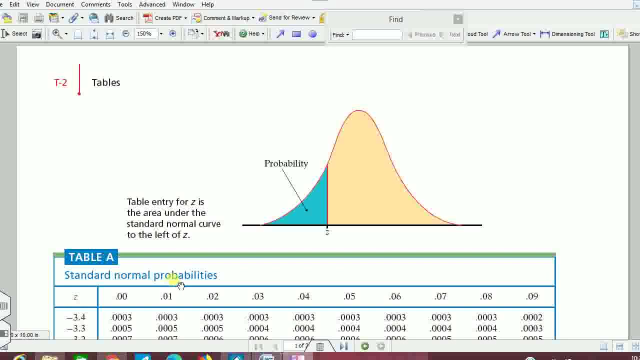 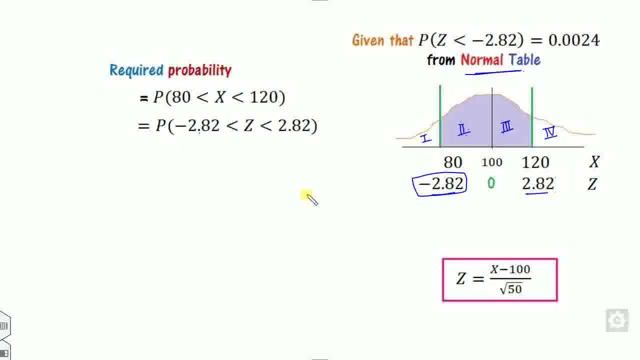 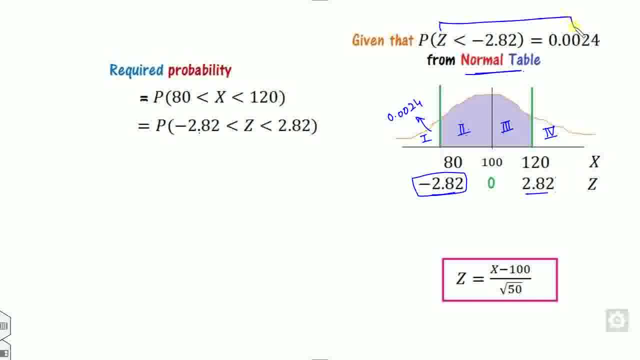 is my 0.0024. i have written here the value from the table. now, once you will get the value of one, can you find the value of the second? yes, you can easily find there is a 0.5 minus of this. can the area of second and third are same? yes, because that what is the length of this is. 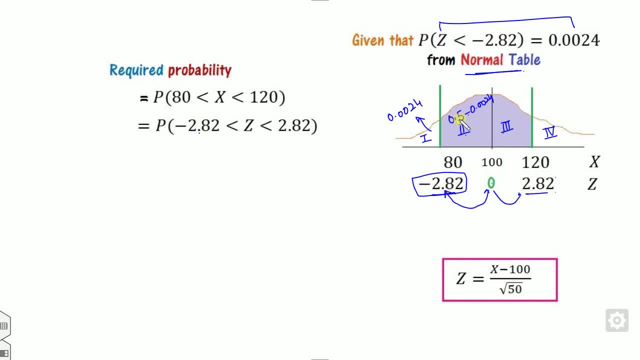 zero to minus 0.2.82, and this is same. so second and third are same. so, therefore, what is the how you find this? how you find this is nothing but here, because all of you know that this value is 0.5 minus of this 0.0024 is nothing but here this is above same, so we can find this value is here. 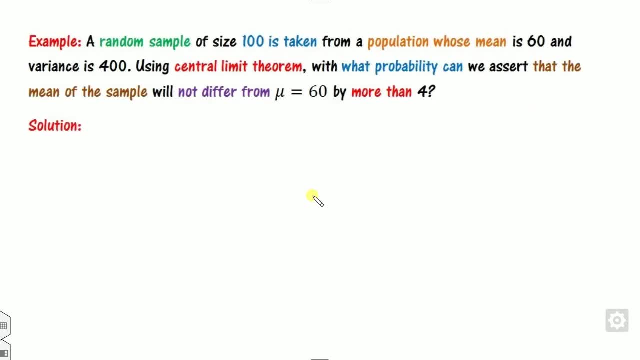 so this is the required answer. now we will look on quickly on the second example. we will do the same thing, same way in this example also, given that n is my 100, so what is given to you? i have written that mean is 160, variance is 400. what is the required probabilities you have to calculate? 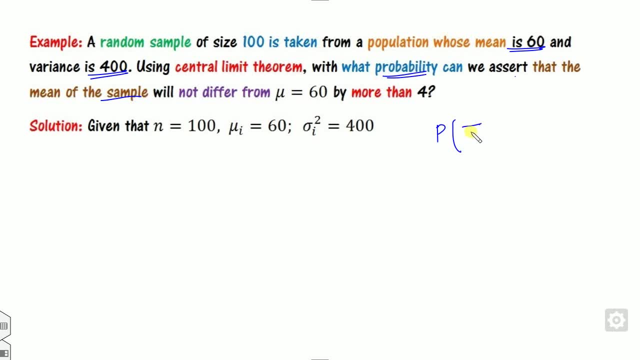 the probability that the mean of the sample- so mean of the sample is denoted as x bar- will not differ by, will not differ by more than 4. that is our task. so our task is to find the mean of this and our task is to find the variance of this. but what is the definition of the x bar? 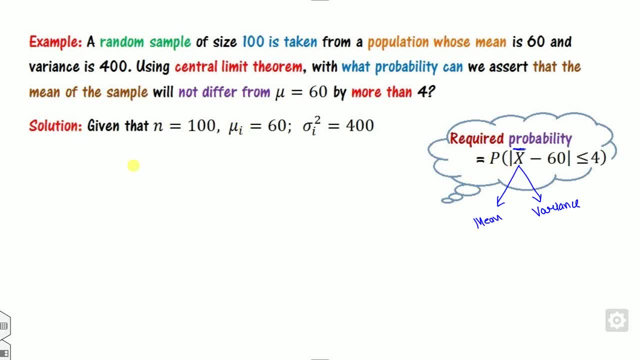 this is the mean of the x. so what is the x bar is here now. our task is to find the mean of the sample. so our task is to find the mean of the sample. so our task is to find the mean of the x bar. we will task is to find the variance of the x bar, and all of us knows that. 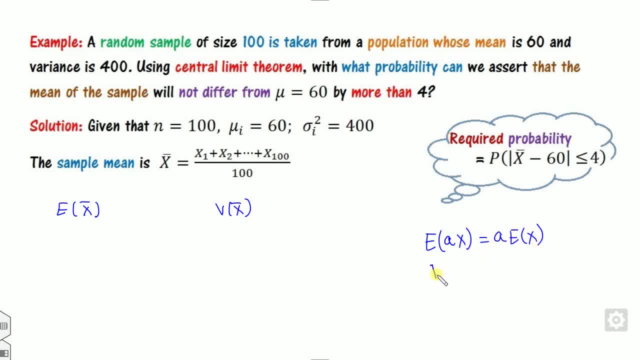 what is the mean of the ax? this is a times of the x. what is the variance of the ax is a square variance of the x. so we can apply here. you can see this: 1 by 100 is a, some summation of this. 1 by a square of this. what is the mean of the xi is 60. so how many times is 100 times? so i can write: 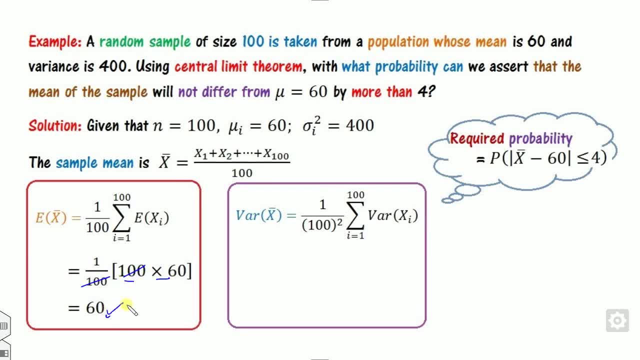 this one as here. so this will cancel out as 60. similarly for this, what is the variance is 400. it's a constant with respect to i. so again, it is a hundred times of this. so 2: 0 will be cancelled out. 400 cancelled out, so 4. 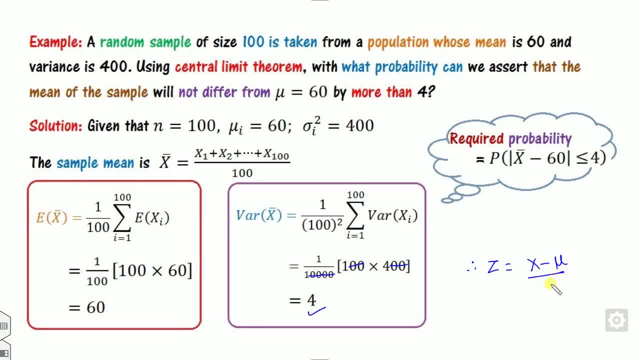 therefore i can define the z like this, so again. so therefore we can substitute the value here: mean is my 60. this is sigma square, so the variance will be my 2, so therefore z will be my here now i can write this on the normal distribution: 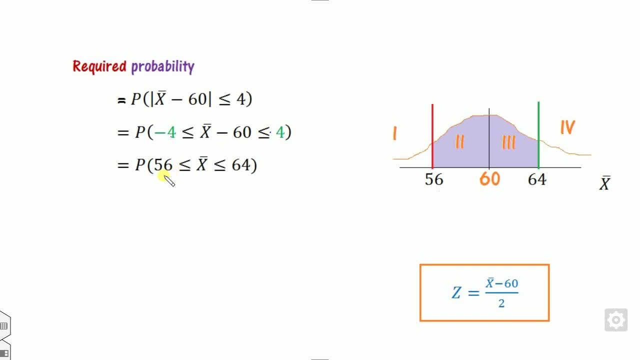 table. i can expand them in terms of minus 4 plus 4. now it's a 56 and 64. i can write here. so again, my areas lies between them. so, corresponding to this x bar, we can define the value of z. so it is 56 minus 60 minus 4, divided by 2, it's a minus of 2, 0, it's plus of 2, so i can write here. 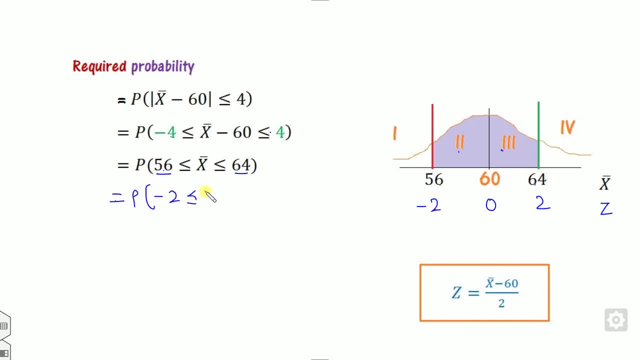 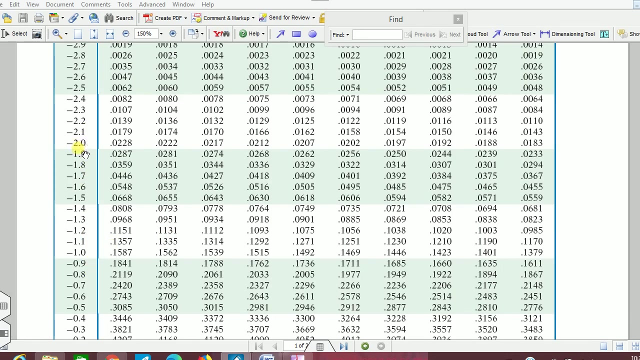 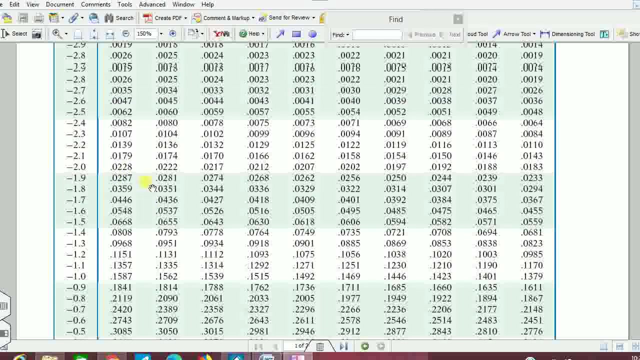 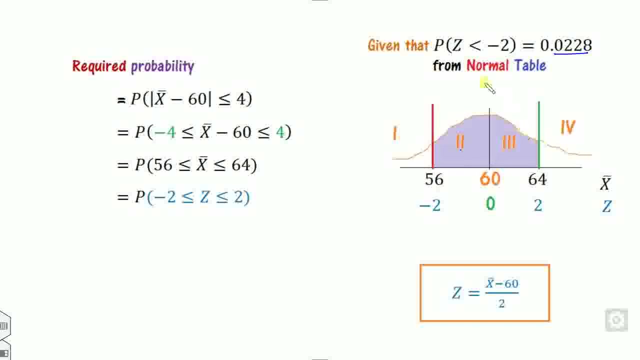 as what is the? 56 becomes minus of 2, x, bar becomes z and it is plus of 2, like here. now my dead sign: thicker if this gets Zed going. i roasted and i wanted to program this value. then i write a like a negative 2 here. so it's three negative power in the half risk. so i 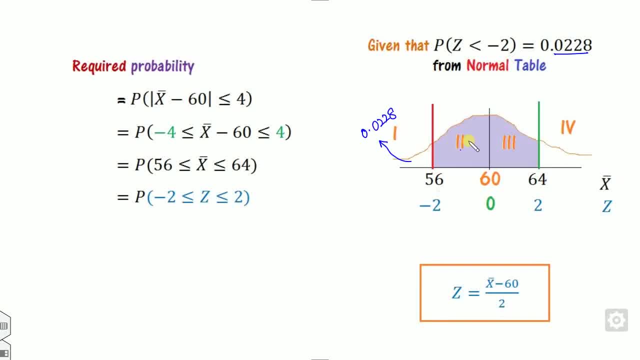 can write it like this: 0.0228 and so on, and so for other observations, you can modify the values. i want to över deliver them with these values so I can process, for example, this is where you have this value bar, so this is where you have to find this value bar and this value bar and close with. we can do that for the α then, and where is the? 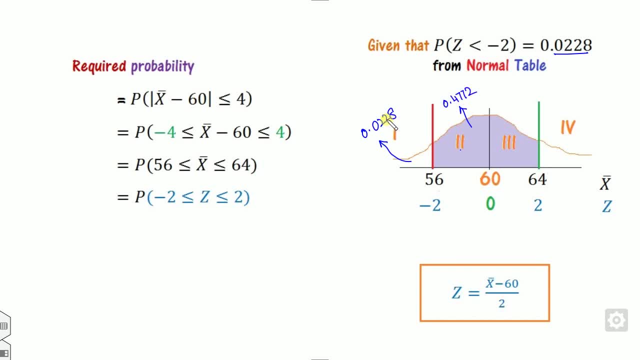 yes, you can find easily the area of second from here. is this 0.5 minus. can area of third be same as that of second? yes, the length is my point. length is my two same, so this is also same. so my task will be this: plus this: 0.4772 plus 4772 is the required answer. so remember our task. 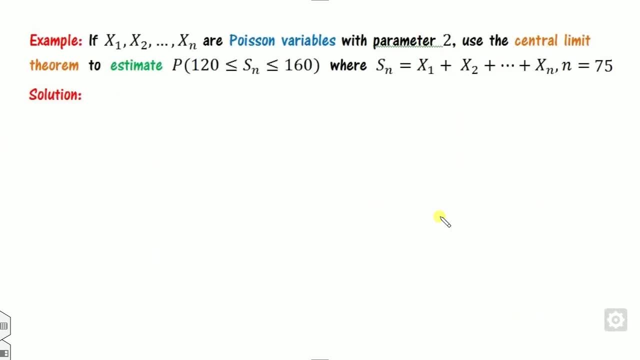 our approach is remain similar. we will do the same approach in each of the way. same method. we will apply here what is given to you. it is a Poiser distribution with parameter lambda. so what is the Poiser distribution is here and how many parameters are there? only one. 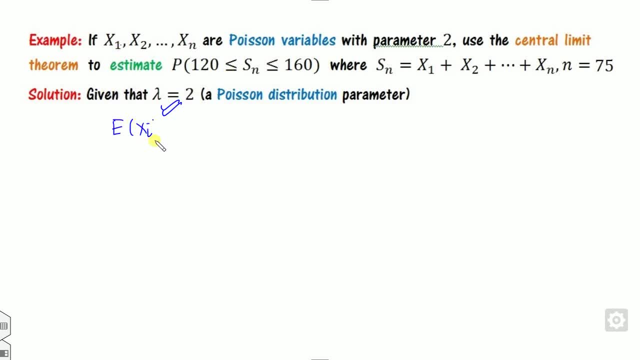 so, therefore, can you find the mean of the excise? what is the mean of the Poiser distribution here? what is the variance of the Poiser distribution is also with this. so you can see the mean and variance are same. now your required task is to here. my task is to find the mean of this. 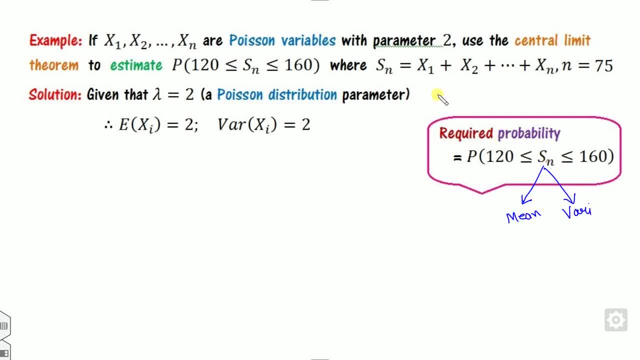 my task is to find the expense period of some value. are these two variables will apply here, the variance of this. so what is the Sn? Sn is here, so therefore I can write: the mean of the Sn is sum of all this. now, n is my 75, so summation will goes to 75, so this will 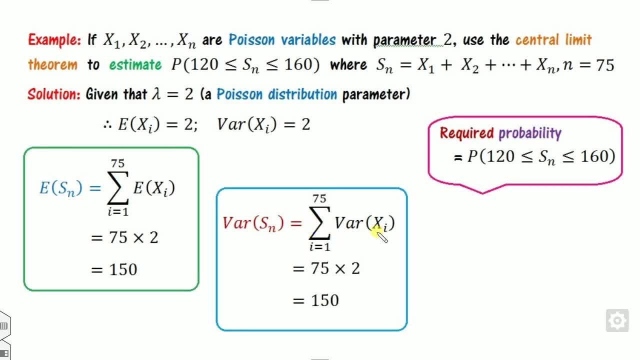 be here. similarly, I can define the variance of this. variance is nothing but here, because all are my independent is there. so 75 into 2. I have to written here as it should be the independent, otherwise we can't open the bracket here. so this is 150 or you can say these are. 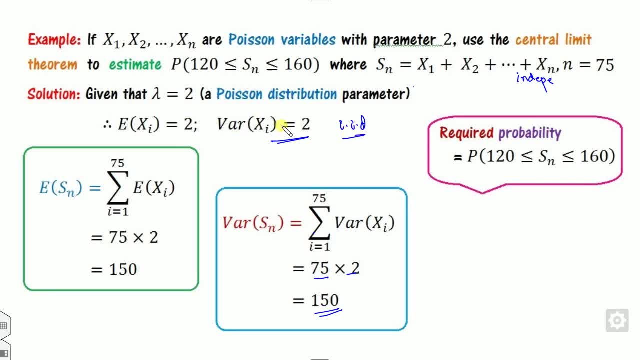 the IID also be, because the mean and variance is both are same for each of the I, so they are IID, so independent is also be there. so therefore, what is the value of the Z is X minus mu divided by Sigma. so this is Sigma. square is 150. so Sigma is here. now we can. 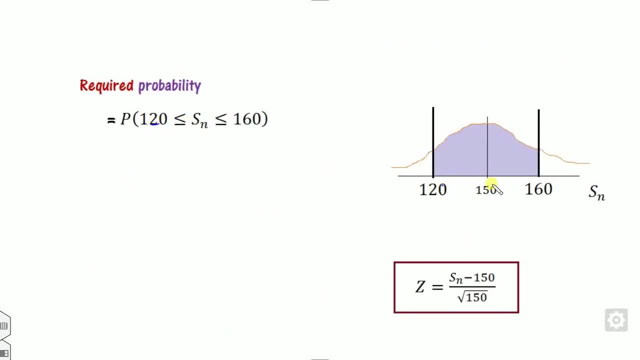 draw the normal distribution curve for them. now. this is 120, 160. I can define the value of Z, so this is minus 35.. this is Z by root. 150. this is G. this is 10 by R150. so if I substitute the value here, 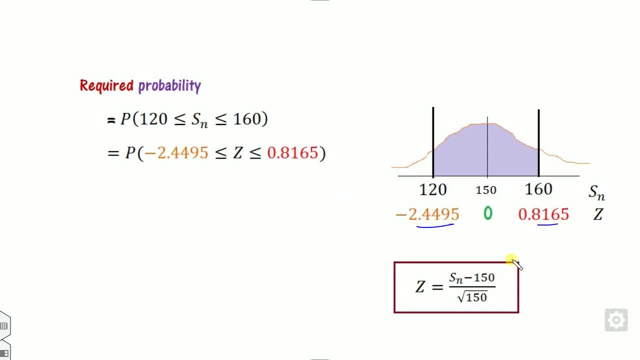 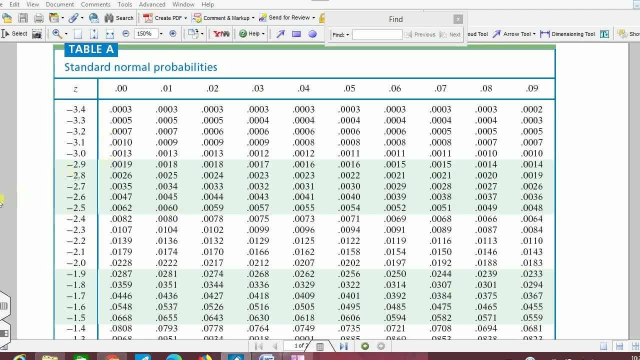 what is our minus 30 by root 50? I can calculate this value here now from the table. we can calculate this value now. but if you see in that table these are up to the 2 decimal places. so what we can do, I can approximate them to be here minus 2.45. what is the value of the? 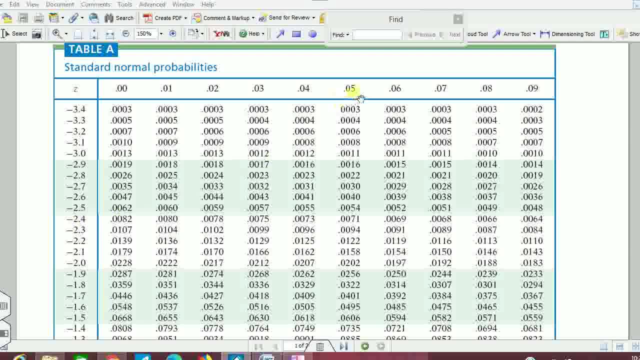 minus 2.45 in the table, minus 2.4 here. 0.5 is here, So the variance will be same for the lp over here at avaliable. And So cinrotouch through the integral, as I said, as I have just shown. 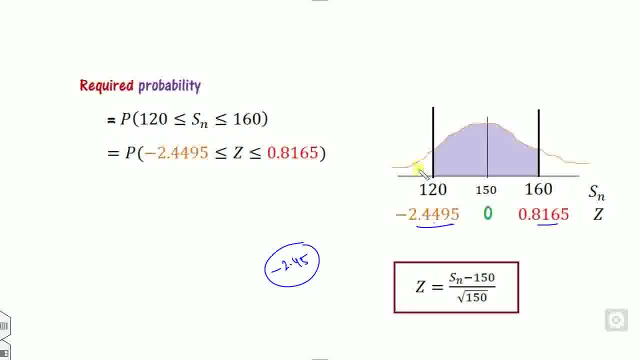 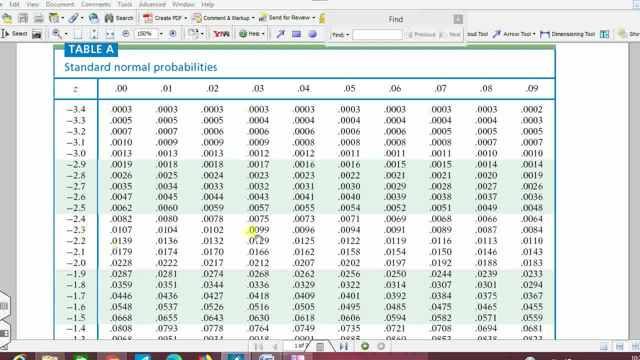 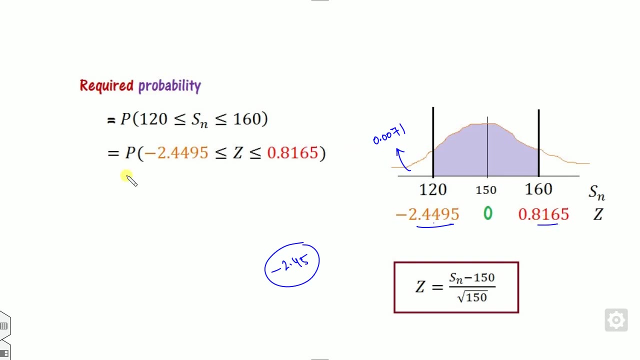 values: 0.0071. it means this value is my 0.0071- look at that again- minus 2.45 and 0.8165, so I can round off as a 0.82 and so on. so I can write this value as here you can see: 0.0. now this will. 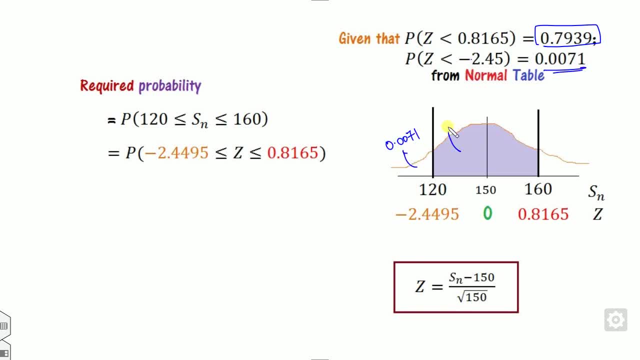 be here: 0.0071. can you find this value easily? yes, you can find 0.5 minus 0.0071, so it will be 0.4929. what is the area of third? now? look at that. this is here, so this is 0.7939, up to this. 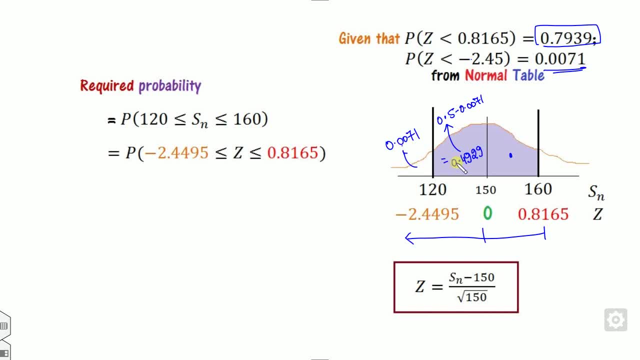 so can you find the area of this? what is the portion of this? you know this part and this 0.5. you can subtract 0.5 from here. you you will get this answer. so what is the required answer? is this: plus of this, 0.4929 plus 0.2939. 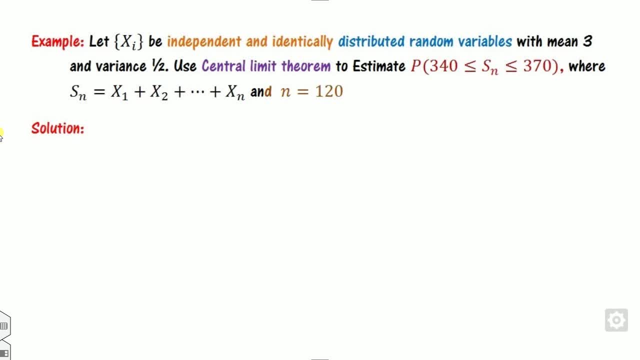 is the required answer. look at the one more example again. we will follow the same procedure. it is given to be independent and identical. mean is 3, variance is half. it means this is given to you. what is my task is you have to find, since n is very large again. so my task is here again. 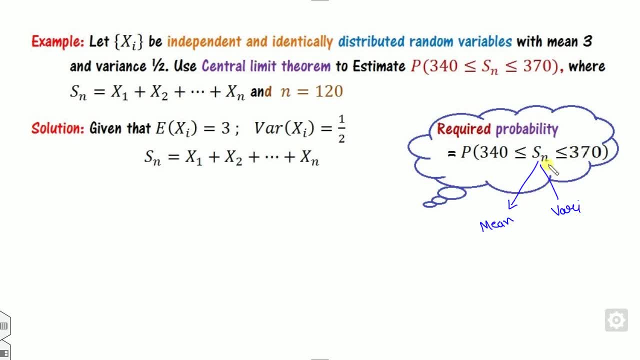 we will calculate the mean. we will calculate the variance for the SN. what is the SN? is this now, in this case, n is my 120, so I can write the mean as i varies from 1 to 120. I can calculate the variance of the SN i varies from. 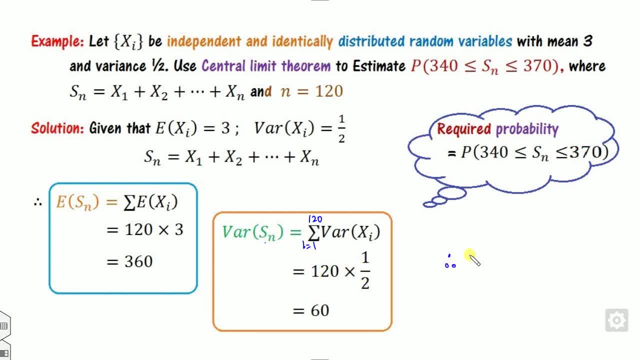 1 to 120 is here, so therefore you can define the value of z again from this. it will be root of 60, because this is the variance and we need the standard deviation. so sorry, this is the standard and we need the standard deviation. so sorry, this is the standard deviation. so sorry, this is the. 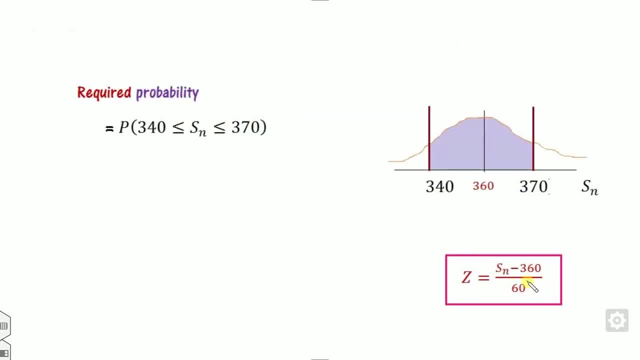 is root of 60. So therefore, we can calculate the value at here. What is the value of this is minus 20 divided by root 60. This is 0. This is plus 10 by root 60. So if I say, this is my area, 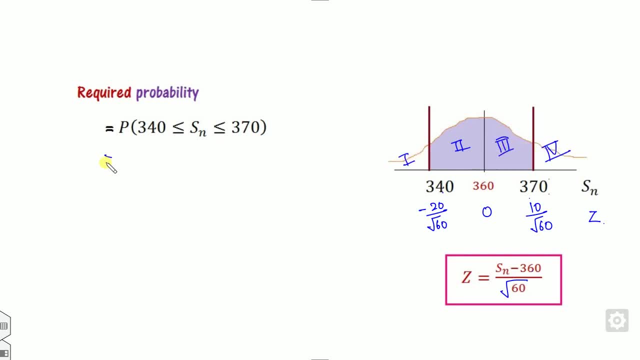 second, this is third, this is four and this is one, So I can replace the value like here. Now again, from the table you can see minus 2.58 if you round off them to be minus 2.5. 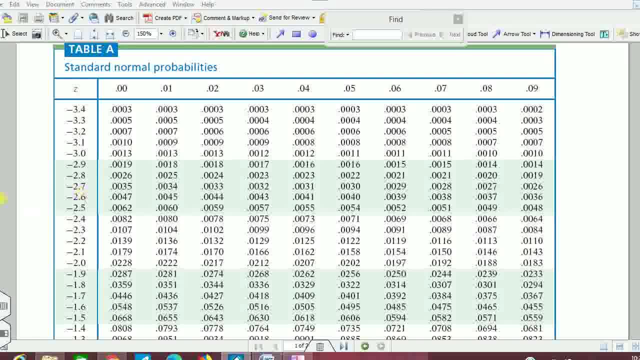 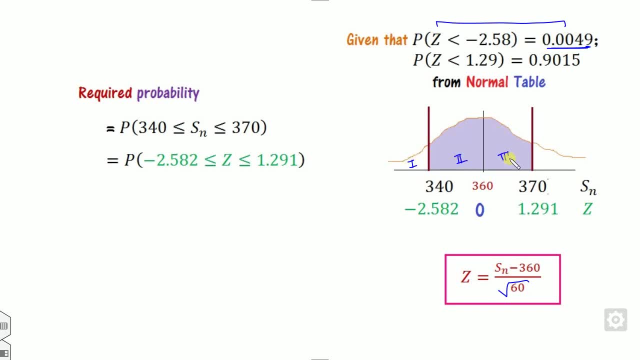 and eight is here 0.0049.. So you can see 0.0049.. So, according to this, which portion is here? Is it 1, 2, 3 or 4?? So this is less than of here. So it means this portion is given to you. 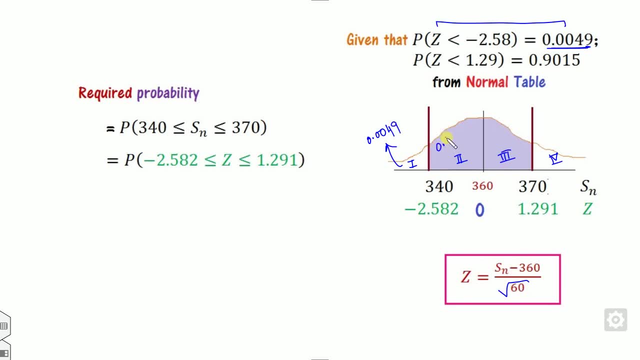 So can you find the area of second: Yes, 0.5 minus of this. So you can write like this way: This is my second. What is this portion? 1.29 approximately, So this will be 1 plus 5.. 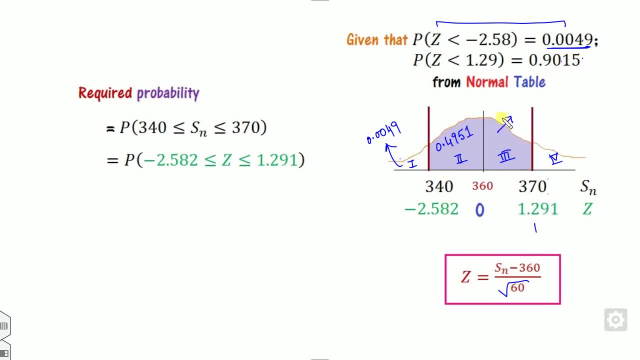 2 plus 3 is here. How you find. the area of second is Area of third is 1 plus 2 is 0.5.. So this is nothing but my here. So what is the required answer? is This plus of this. 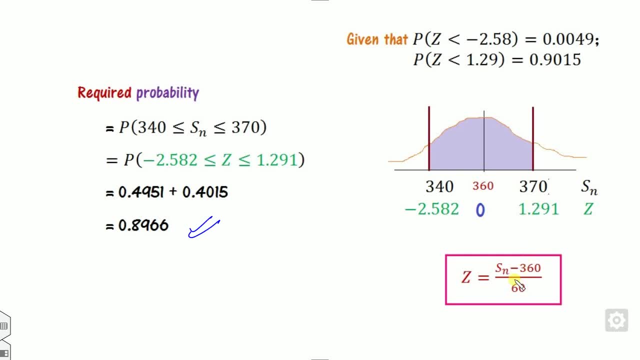 is the required answer. So this is the way you can solve the any of the central limit theorem. Make sure that you have to follow the same rule, that is, you have to find the mean and variance and then draw the graph. We will see some more lectures related to the central limit theorem.